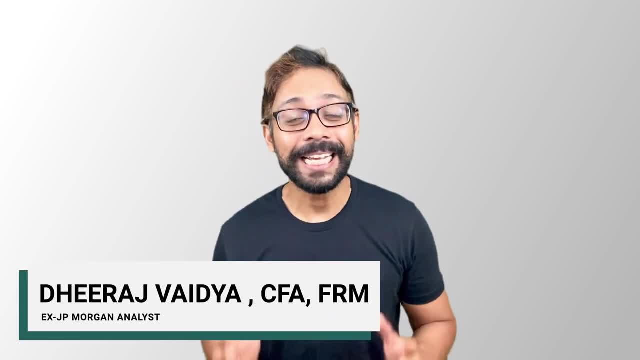 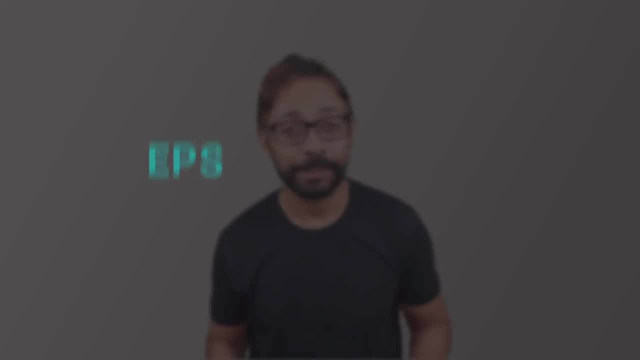 Hi all, my name is Dheeraj from wallstreetmojocom, And in today's video we'll learn all about diluted EPS: what it is, how it is calculated and how it is used. So let's get started. 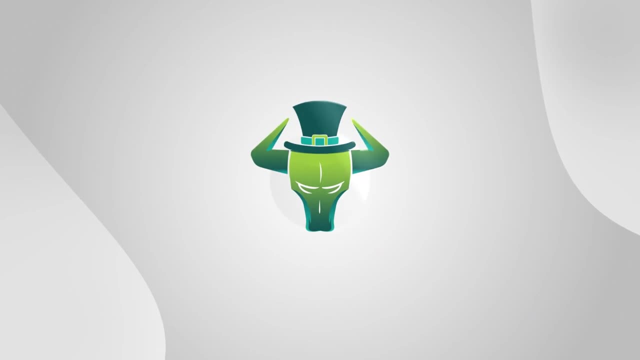 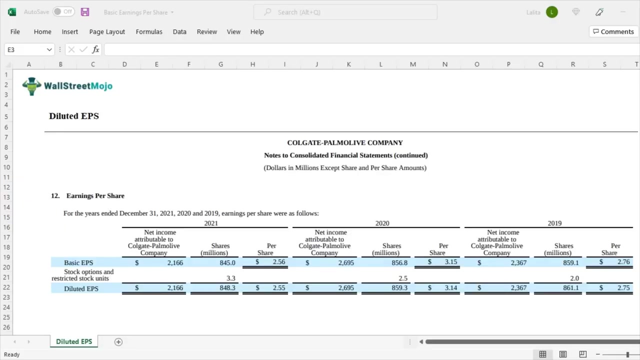 So, before we get into the detailed discussion of diluted EPS, first and foremost I would like you to get an intuitive understanding of what it means. So for that, I would like you to look at this 10K earnings per share data from Colgate-Palmolive. 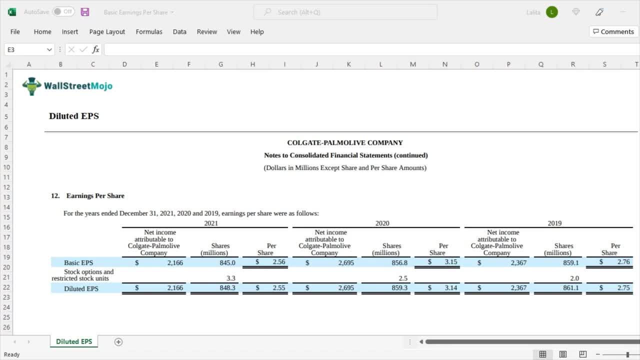 Now we have three years of data: 2021, 2020, and 2019.. Okay, And when you look at this earnings per share or the eps data, closely, we are provided with two kinds of eps: one is the basic eps and the other one is the diluted eps. so if you are new to the basic eps or the 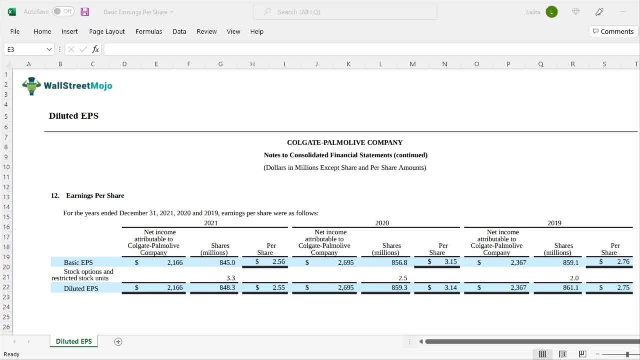 earnings per share overall concept, then please refer to our video earlier, which we have made as a comprehensive video discussing all of these concepts. but let's assume that you know what basic eps is and let's see how the calculation goes. you know, this is the net income, 2166 and the 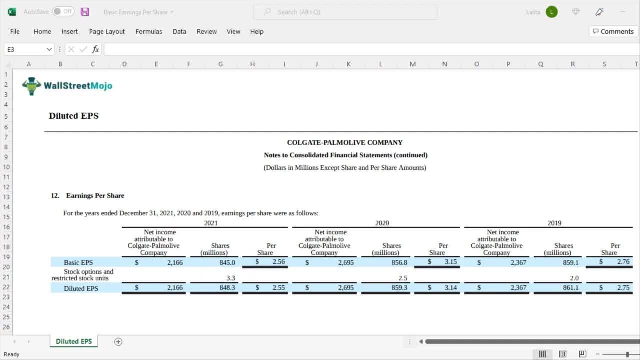 total number of shares outstanding is 845, so what we get is 2.56. now, visually, if you look at, what's the difference between basic eps and the second one, that's, the diluted eps? is it in the numerator? no, is it in the denominator? of course, yes, because we see that there is something that's called as: 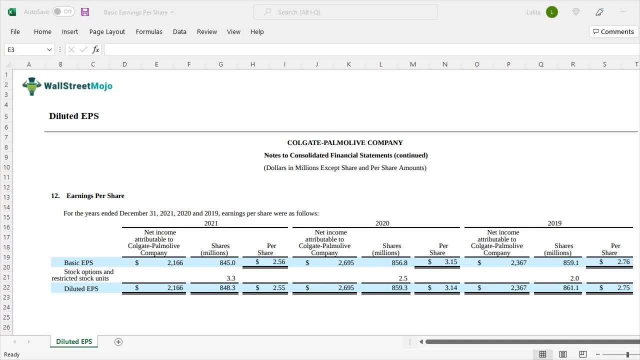 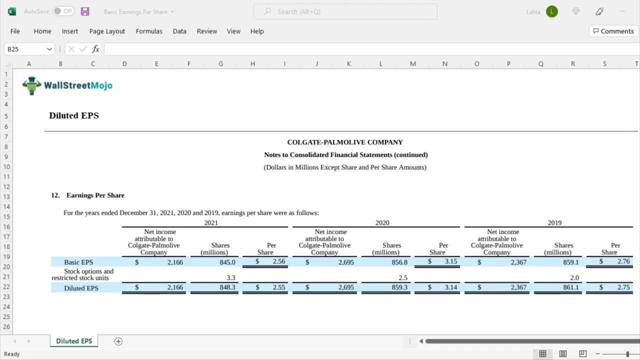 stock options and restricted stock units. that's the difference between basic eps and the second one, that's the diluted eps that have been added to the denominator. so, essentially, the denominator increases from 845 to 848.3, thereby reducing your eps, and that's why it's called as a diluted eps. so the difference 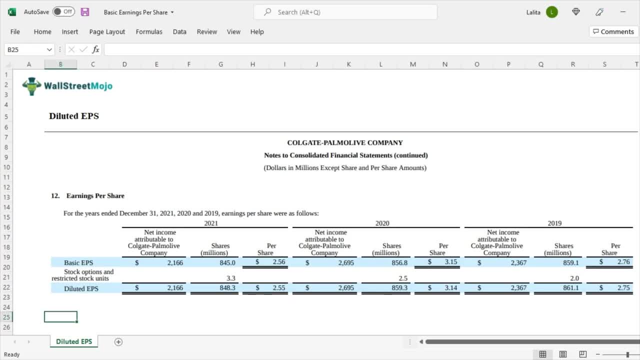 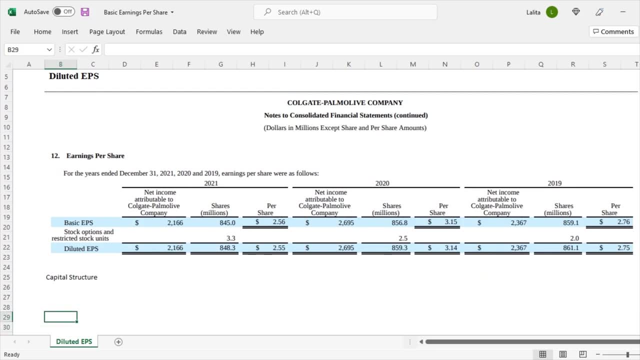 between the basic eps and diluted eps comes primarily from the capital structure of the company. okay, and the capital structure of the company can be divided basically into two parts. the first one is the simple capital structure, and that consists of common shares, or the ordinary shares, and the preferred shareholders as well. okay, 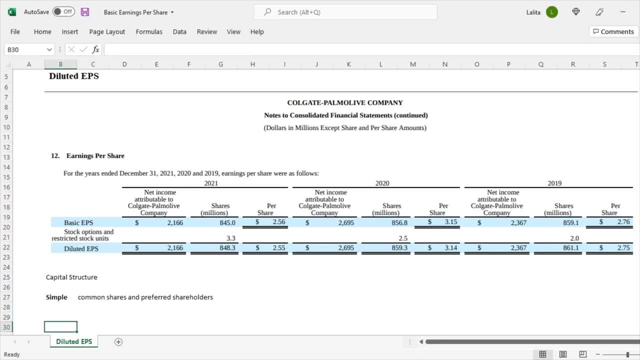 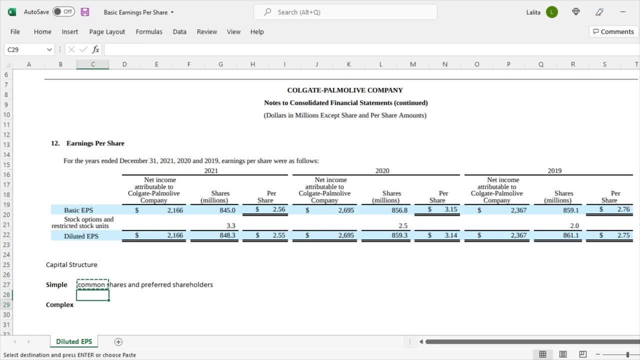 so that is called as a simple capital structure. the second one is the complex capital structure. so the complex capital structure not only has this common shares and preferred shares, but it also has things like stock options, um restricted stock units and, you know, convertible debts. so these securities 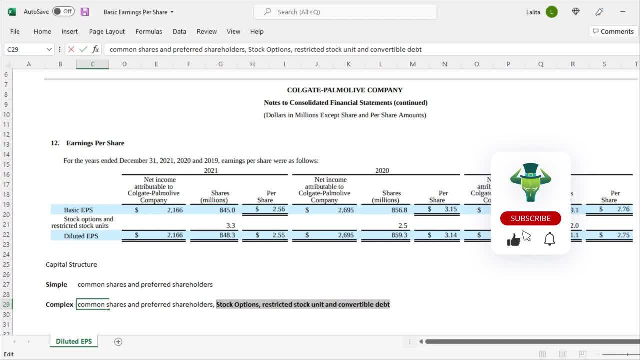 which i have added here: stock options, restricted stock units and convertible debts. they essentially lead to, you know, formation of more number of shares over a period of time, and that leads to the dilution. so let us look at stock options here. so stock options are the options which the company 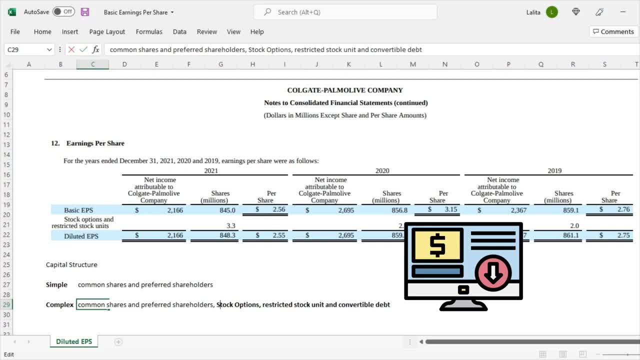 gives to its employees. all right. so it allows the employees to basically purchase the stock of the company at a price which is lower than the prevailing market price. so if you look at the, So essentially this technique is used by many companies to retain the top employees for the 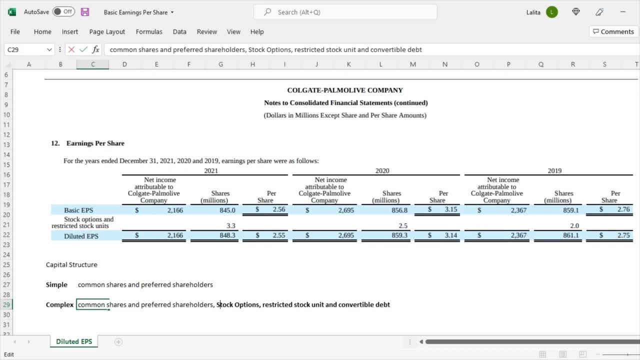 long run. but the overall effect on the number of shares is that when they exercise their options, the total number of shares will increase. So likewise, think of restricted stock units. Restricted stock units are nothing but actual shares which will be given to the employees if they stay in the company for a certain period of time. Next comes the convertible debt, So in 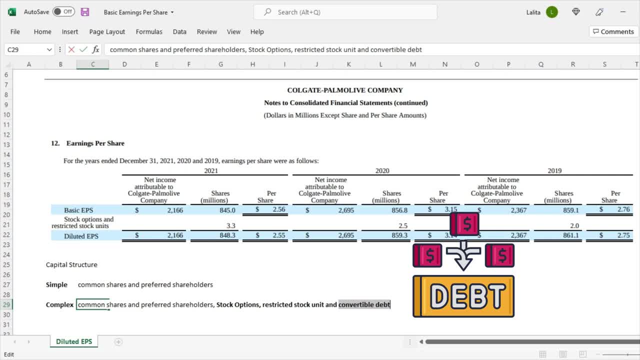 convertible debt. what happens is that this form of debt can convert into actual shares at a predetermined price. So when it happens, the overall number of shares will increase, So that again leads to dilution. So essentially, when your capital structure is complex, you will have an. 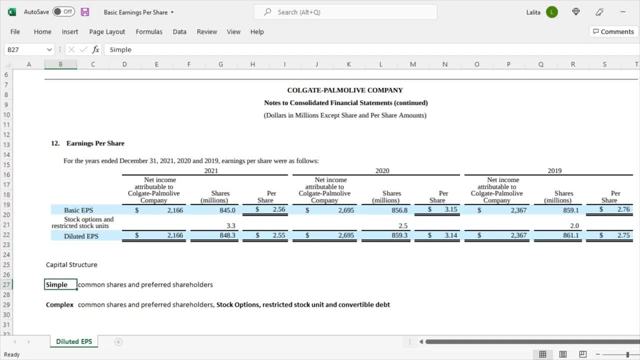 existence of diluted EPS. But when you have an existence of diluted EPS, you will have an existence of diluted EPS. So if you have a capital structure which is only simple, then your basic EPS and diluted EPS will be one and the same, because there won't be an effect of stock options and restricted stock units. and 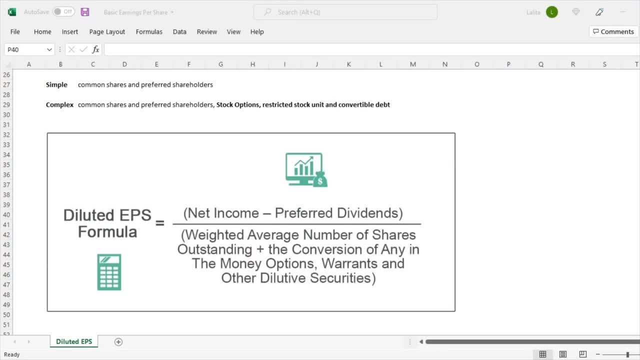 convertible debts altogether. So now let us look at the formula of diluted EPS. So let's look at the numerator. first, Net income minus preferred dividends. So this remains same For the basic EPS as well as for the diluted EPS. both of them remains the same. In the denominator, there's only 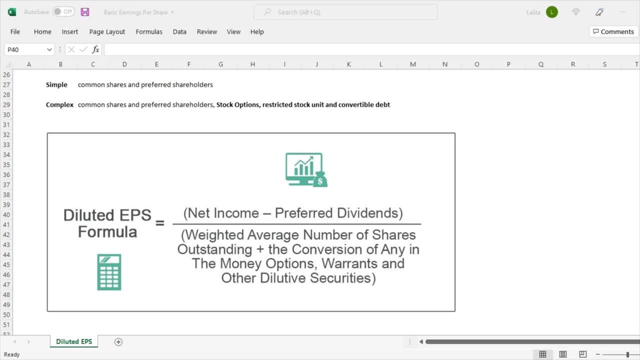 one change. The change is that if you have a capital structure, which is only simple, then your first is the weighted average number of shares. That remains the same, But the change is that you need to add any conversion that happens because of stock options or restricted stock units, or 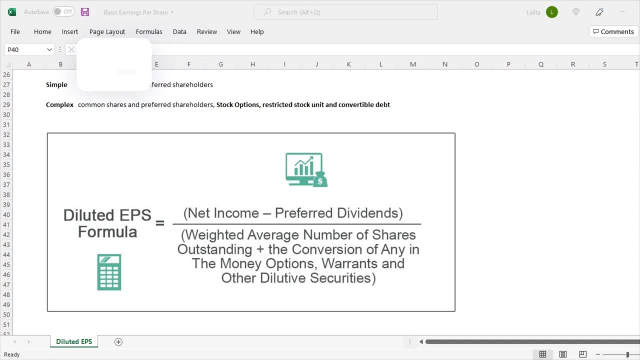 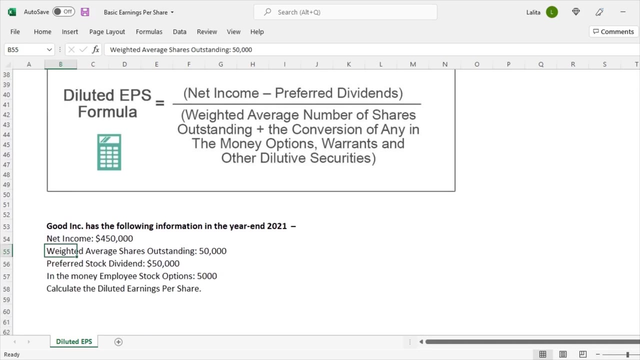 convertible debts into the denominator. So that's the only change. So once you add this up, you will get a higher number from the total number of shares outstanding point of view, And this will result in a diluted EPS. Let us now look at a very basic example of diluted EPS calculations. 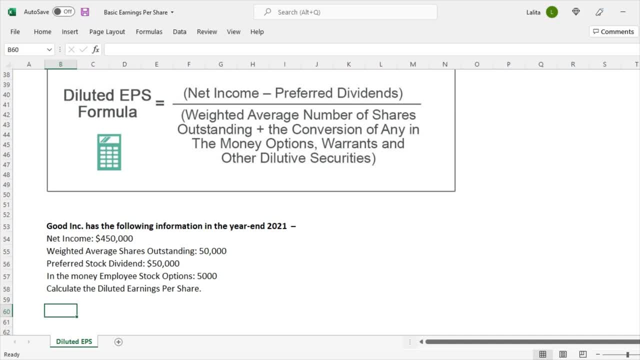 So here we have a stock option, which is only simple. So let's look at the denominator. So let's look at the basic EPS. We have this good incorporated company who has provided us with the data of 2021.. So we have this net income as $450,000.. Weighted average number of shares outstanding is $50,000.. Preferred. 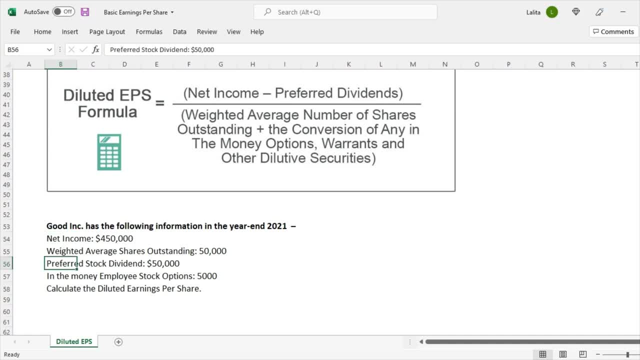 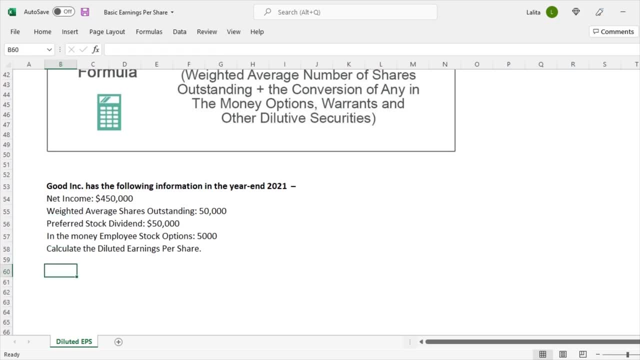 stock dividends is $50,000 and in the money, employee stock options is $5,000.. So we are expected to calculate the diluted earnings per share. Okay, so let's first, you know, calculate the basic EPS. What is the basic EPS? Basic EPS is nothing but net income minus. 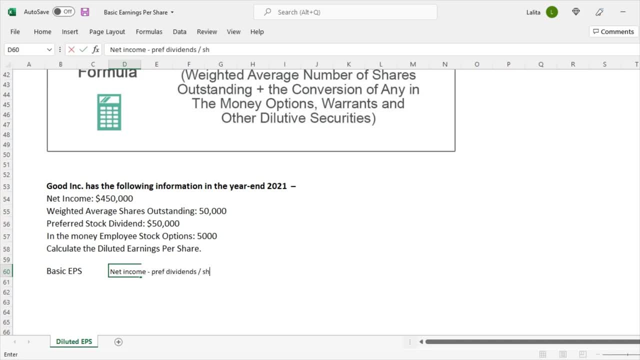 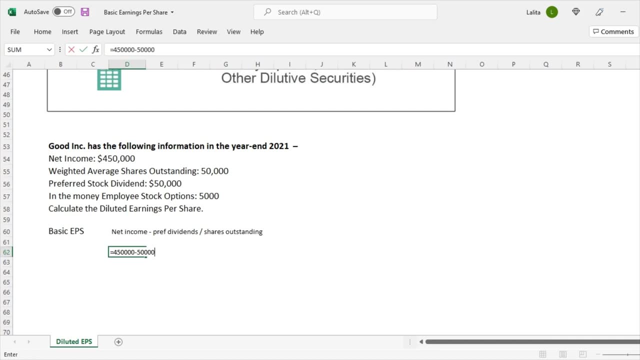 preferred dividends divided by the shares outstanding, right? So this comes out to be net income for $50,000, minus $50,000 as the preferred stock dividends. So the numerator is $400,000, and this total divided by your total shares outstanding, that is $50,000. right, So we get. 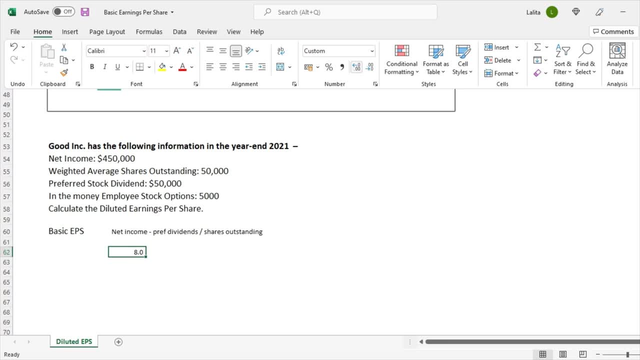 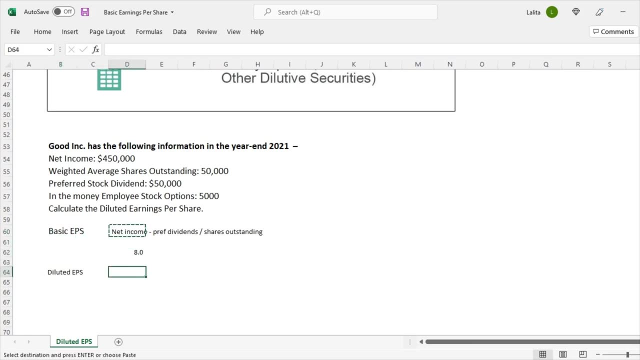 the basic EPS as 8.00. right, So let's calculate the diluted EPS now. So let's calculate the diluted EPS now. The formula for diluted EPS in this case will be net income minus preferred dividends divided by your shares outstanding. and since we have only one dilutive security, that is in the money stock. 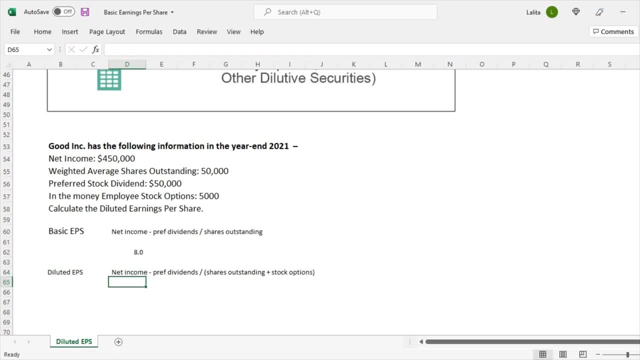 option. So we'll write this as stock options. okay, dilution. So let's calculate that Here the numerator will remain the same: $450,000 minus $50,000, and divided by your shares outstanding, That is $50,000. and we need to add the effect of dilution as well, that is $5,000. okay, So we get. 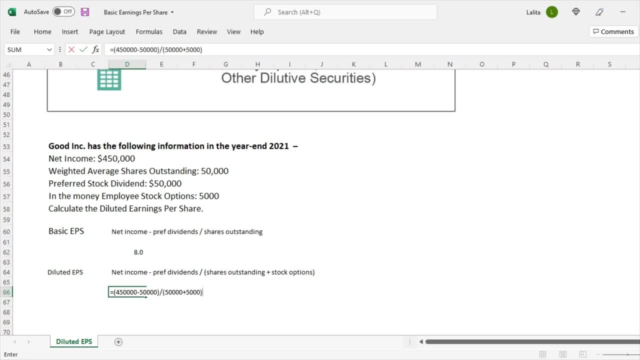 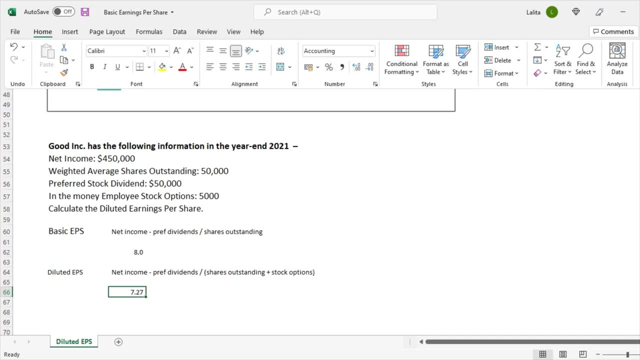 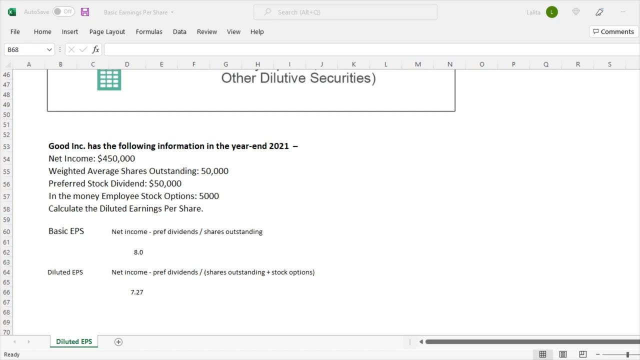 this as $55,000 as the denominator, So the total diluted EPS will be 7.3, or that is 7.27.. Okay, so this is how your diluted EPS can be calculated. So, as a quick note, I just wanted to tell you that the formula that we have learned is not fully robust, and 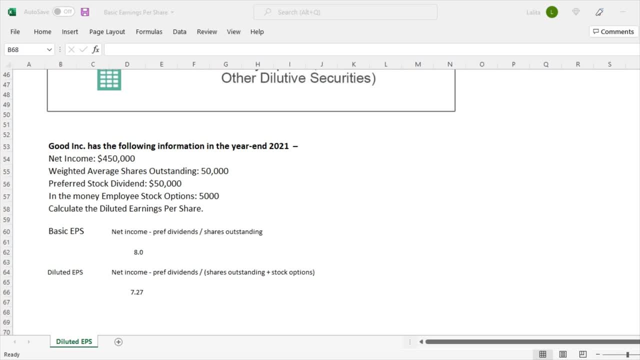 there are certain limitations of the formula that we essentially used. So what I meant was that, as an analyst, if you're using it, there would be certain adjustments that you are expected to do. So think of convertible debts, for example. you know, When you look at convertible debts, 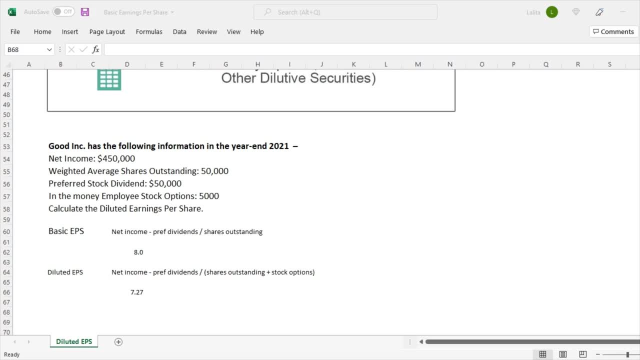 so in the denominator you might want to add the number of shares because of the convertible debt, but because of that you might be saving the interest, right? So you have to adjust the numerator as well. So these small adjustments I haven't discussed yet. Likewise, 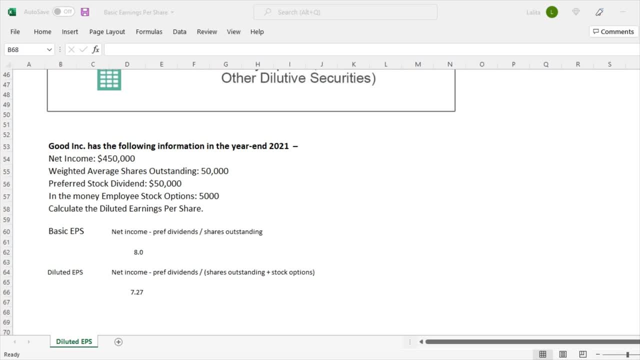 how do we calculate the in the money stock options? So if there are hundred stock options, out of which how many are in the money? So you basically use treasury stock method to do that. We haven't discussed that here yet. Okay, so that's the limitation of this whole calculations. Another: 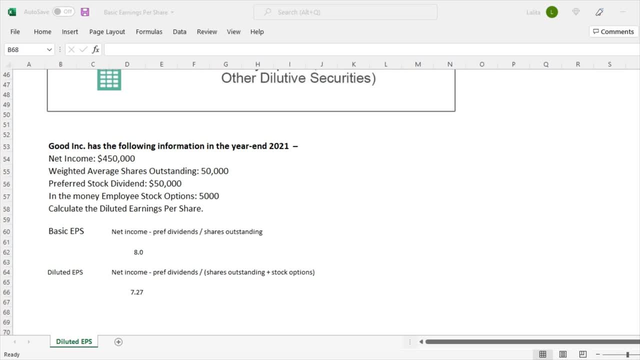 thing is that you know if there is something called as a convertible preferred shares- So convertible preferred shares are different from preferred shares- These convertible preferred shares would mean that they might convert into actual common shares. So if that happens, then how the adjustment happens, right, You know there would be two effects. 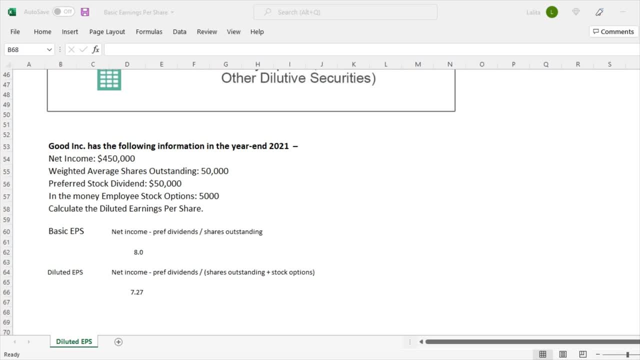 One is that in the numerator you would like to add back the dividends which are there, and in the denominator it will lead to the additional number of shares altogether. We haven't discussed that yet. So likewise there is this concept of anti-dilutive securities. So all the things which 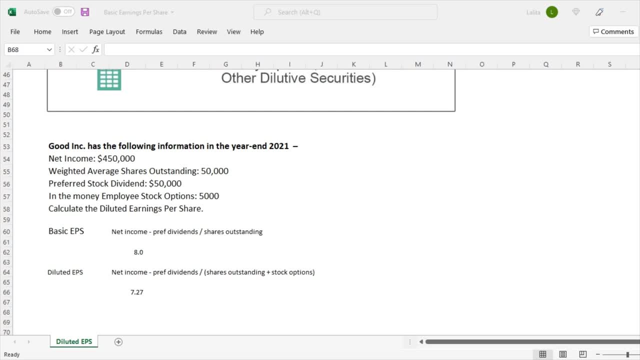 we have discussed right now, it can lead to increase in EPS as well. So if that happens, you don't have to worry about that, You can just go ahead and add it in the calculations. Okay, so we didn't discuss that too. So here this is a very basic example which we have taken, and all the advanced 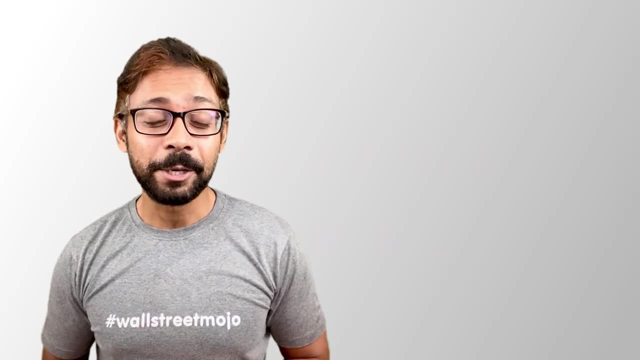 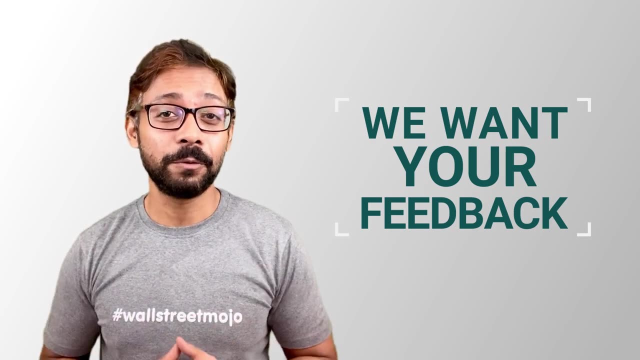 adjustments have not been taken yet. This is the limitation of the whole discussion altogether. I hope you found this video to be useful. Please do like and share, and if you have any feedback or want to suggest a topic for any future videos, then you may do so by writing about it in the. 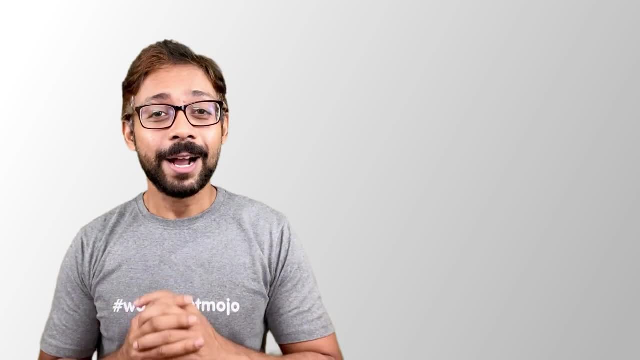 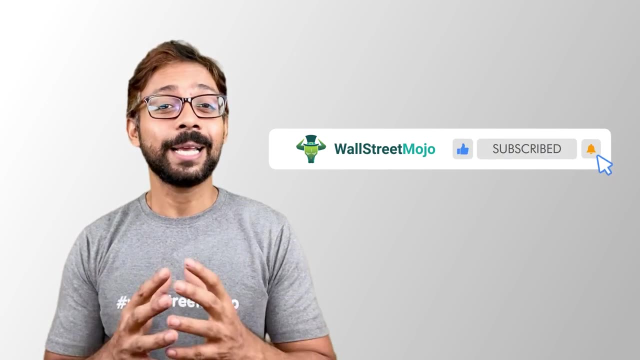 comment section. Also, we come up with interesting videos on finance and accounting. So if you have not subscribed to our channel yet, then please do so by clicking on the subscribe button, so that you can get the notification as soon as we release the new video. Thanks for watching. Have a nice day. Have a nice day.